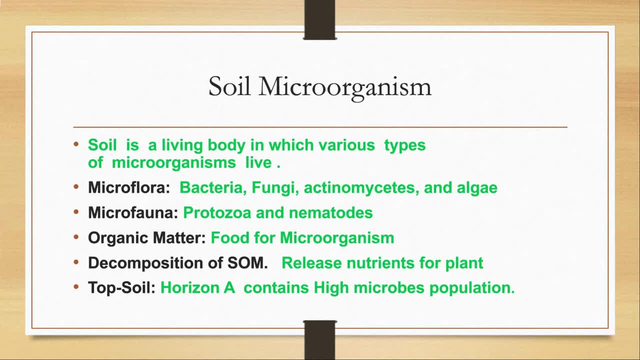 Swale microorganisms are divided into two groups: microflora and microfauna. Bacteria, fungi, algae and actinomyces are all microorganisms. seeds are micro flora and they play a major role in decomposing of soil organic matter. 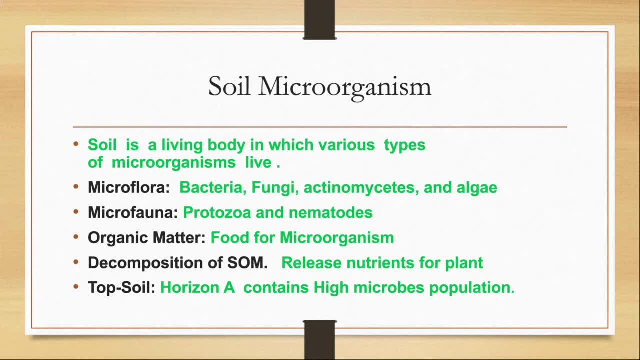 while protozoa and nematodes are micro fauna. protozoa play an important role in mineralizing nutrient and they are free living. they regulate number of the bacteria. however, nematodes cause diseases in plants. they are very harmful microbes for the plants while soil contains organic matter. 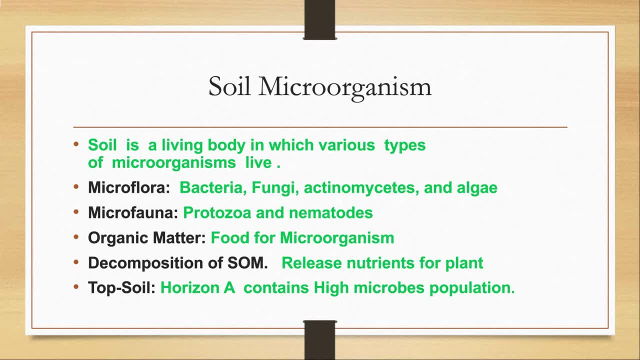 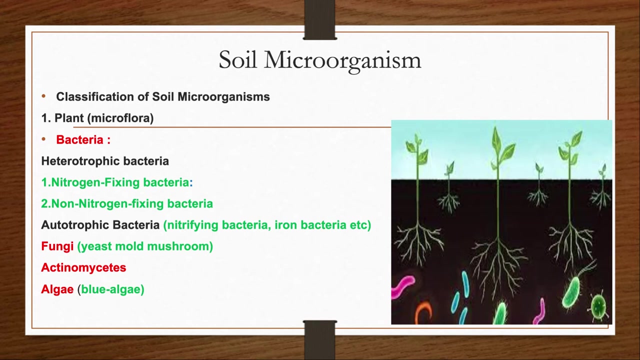 that is food for microorganisms. soil microbes decompose raw organic matter into humus and thus release nutrients in plants. available form: top soil has a high microbial populations because top soil contain higher amount of the organic matter. classification of soils: as i told you, soil microbes are divided into two groups: micro fauna and micro flora. 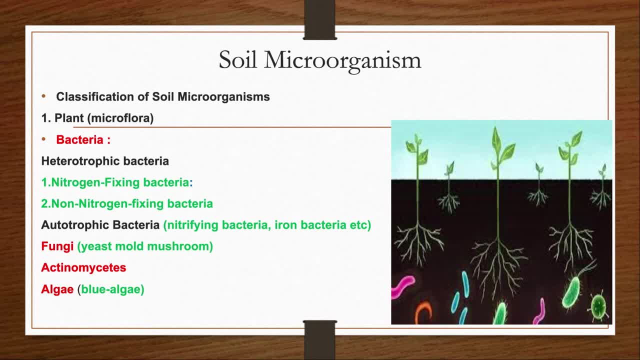 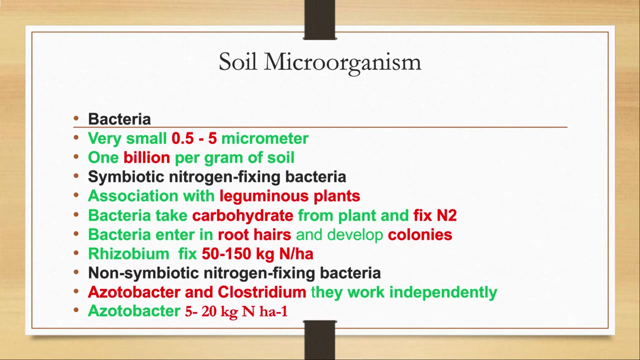 micro flora includes the bacteria, fungi, algae and actinomyces. there are two types of bacteria in soil: heterotrophic bacteria and autotrophic bacteria. heterotrophic bacteria are divided into nitrogen fixing bacteria and non-nitrogen fixing bacteria. let's discuss each of soil micro flora in detail. bacteria bacteria are very small. in size ranges from: 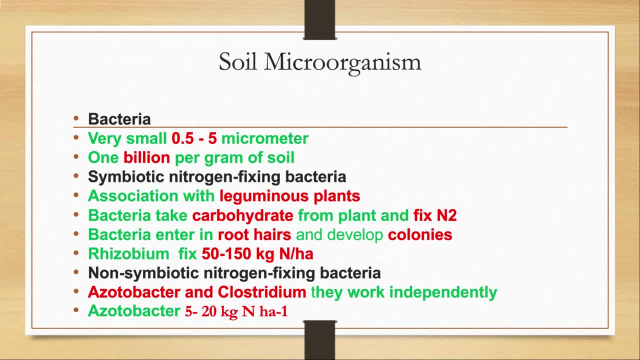 five to five meters. they are most abundant in soil. one teaspoon of soil contains one billion bacteria. can you imagine one billion or up to one billion? most of bacteria are very important for soil and plant. while some causes disease, the heterotrophic bacteria depend upon soil, organic matter, our living body, for their food. bacteria fix atmospheric nitrogen into the plants. 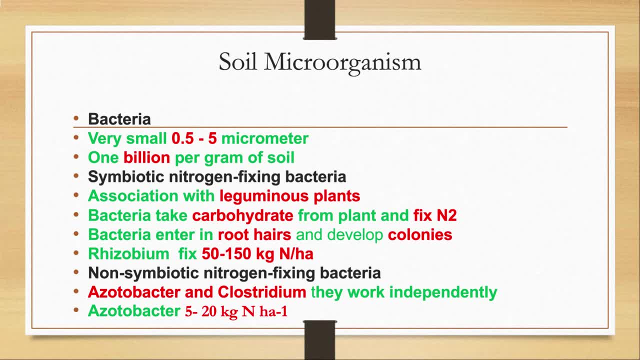 available form. in atmosphere 78 nitrogen is present. that is elemental form and not plants. available form. plants are unable to take elemental nitrogen, so microbes fix elemental nitrogen into plants. available form nitrogen fixing bacteria. there are two types of nitrogen fixing bacteria: symbiotic nitrogen fixing bacteria and non-symbiotic. 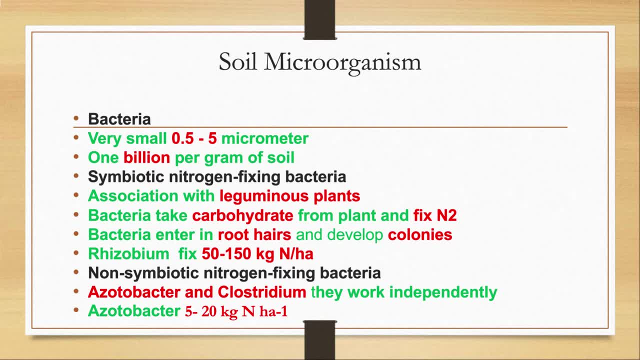 nitrogen fixing bacteria rhizobium. rhizobium is a symbiotic nitrogen fixing bacteria. they fix nitrogen in the association with leguminous plants. symbiotic means interaction between two different organisms. rhizobium bacteria enter in the root of plant and take carbohydrates from plant root tissues. 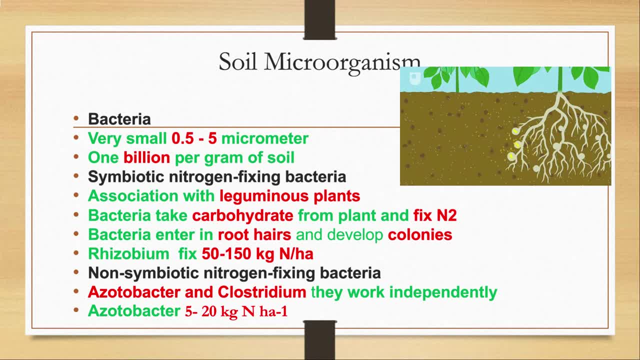 as their food and fix nitrogen in the plant. and they fix nitrogen in the plant using the help of nitrogen, and then they fix the nitrogen in the plant, as well as by using the help of nitrogenized enzymes. rhizobium develop colonies in the plant roots and form small nodules. 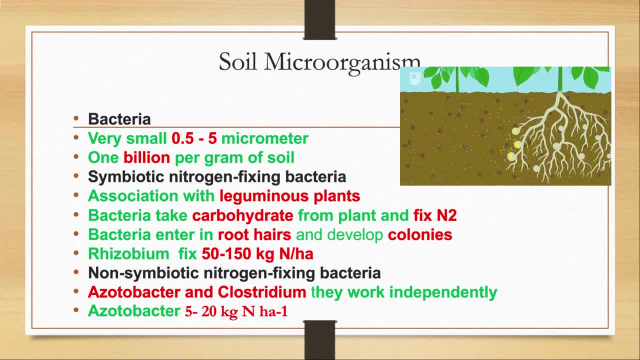 in this symbiotic relationship, both species get benefits. bacteria take their food from plants roots and give fixed nitrogen to the plant, while through this process, rhizobium bacteria fix 50 to 180. Bacteria fix 50 to 150 nitrogen per hectare on symbiotic nitrogen fixing bacteria. 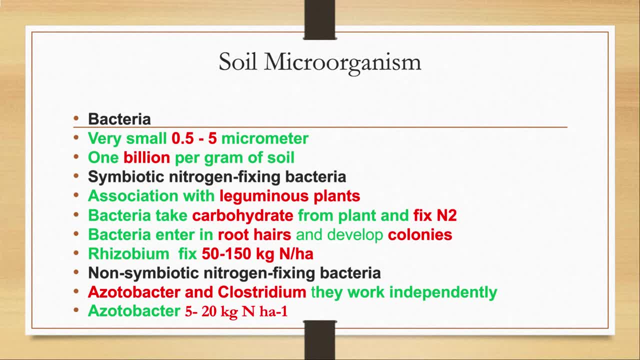 They fix nitrogen in rhizosphere, but these bacteria do not need plants roots. They fix elemental nitrogen into plant. available form examples are Azotobacter and Clostridium. Azotobacter works in the presence of oxygen, while Clostridium is an anaerobic. 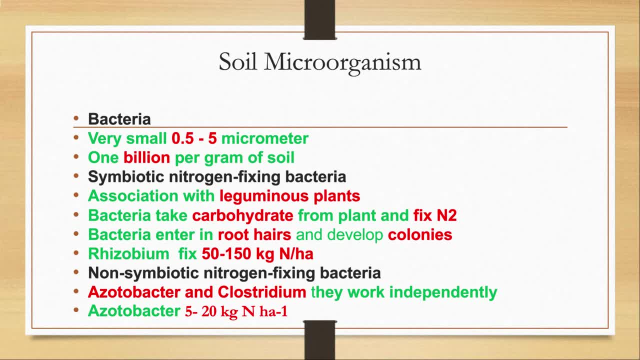 Bacteria. they do not need oxygen. They can work without the presence of oxygen. These bacteria depend on organic matter of soil. They require higher amount of carbon, while azotobacter fix 5 to 20 kg nitrogen per hectare. Decomposition of organic matter by microorganisms. 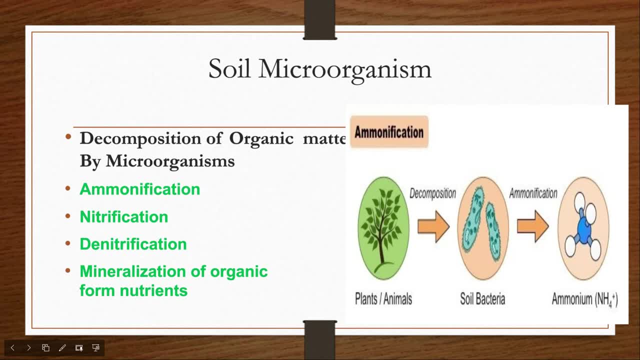 Soil bacteria decomposed organic matter and involved in various problems such as ammonification, nitrification, denitrification and mineralization of organic form of nutrients. Non nitrogen fixing bacteria are involved in these processes. They do not fix elemental nitrogen, but they ammonify, nitrify and denitrify nitrogen in soil. 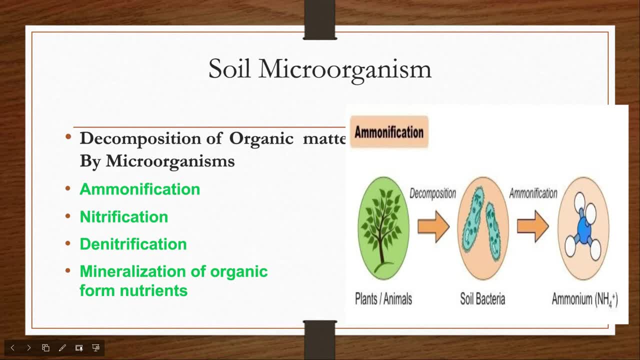 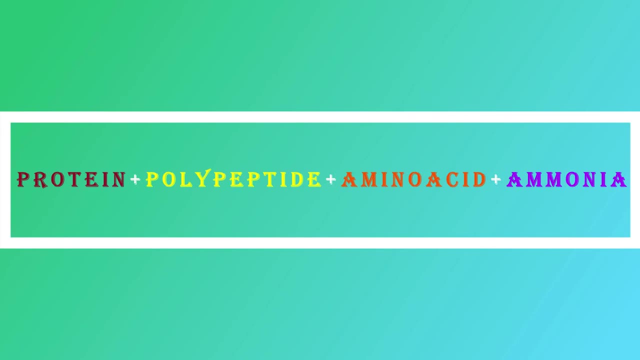 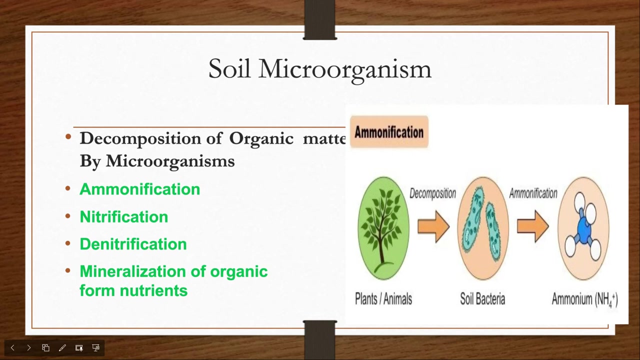 Ammonification is the process of changing organic nitrogenous compounds into the ammonia. in this process, Ammonifying bacteria convert nitrogenous compounds of organic matter, such as a protein, into polypeptides, Then into amino acids and then into ammonia, while in nitrification, nitrosomonas bacteria converts ammonia into nitrite and 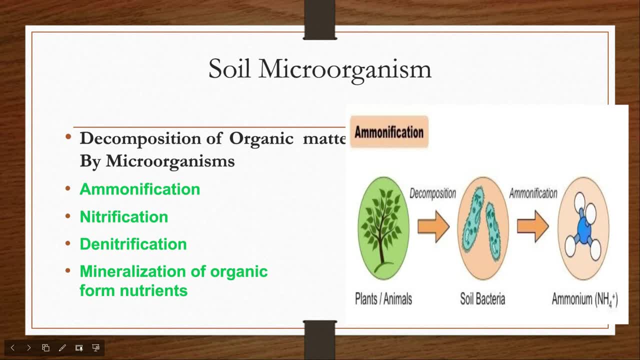 Then nitro vector converts nitrite into the nitrate. Nitrous is also available form of nitrogen for the plant, While denitrification is a process in which nitrate converted into nitrogen gas. in this process, Cytosomonas and Bacillus bacteria are involved. 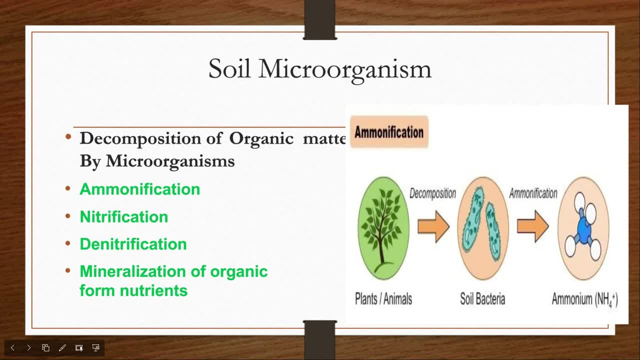 Mineralization of organic form of a nutrients into the. in organic form in soil there are autotrophic bacteria and these bacteria oxide certain nutrients into the plant. available form as microorganism of Oxide sulfur into the sulfate and that is available form for the plant. 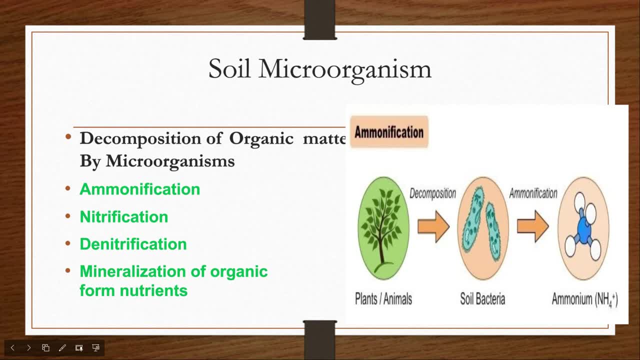 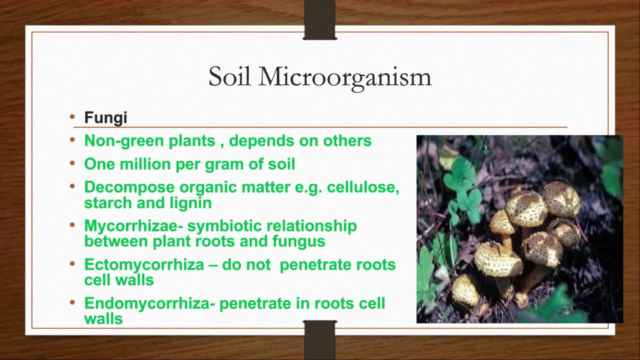 While microbes mineralized organic phosphorus into the plant available form of the phosphorus, fungi fungi, also called fungi fungi, are either multicellular or unicellular. They are categorized as a microorganisms. They depend on other for their food. Do you know? one gram of soil contains 1 million fungi. 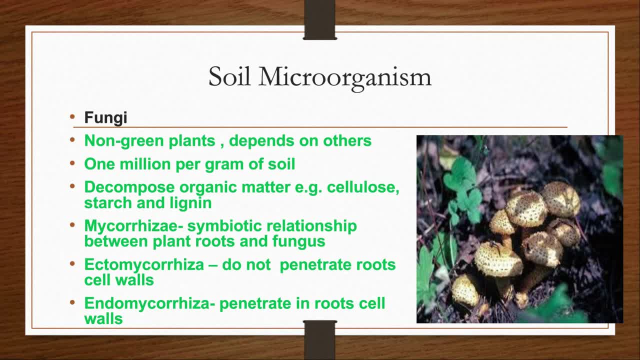 fungi decompose while organic matter and very hard materials such as cellulose and lignin. fungi make Symbiotic relationship with a plant's root. that is called my crazy. That is a mutually beneficial association between certain fungi and roots of plants. in This symbiotic relationship are in this symbiotic association, fungi get sugar from the plants root. 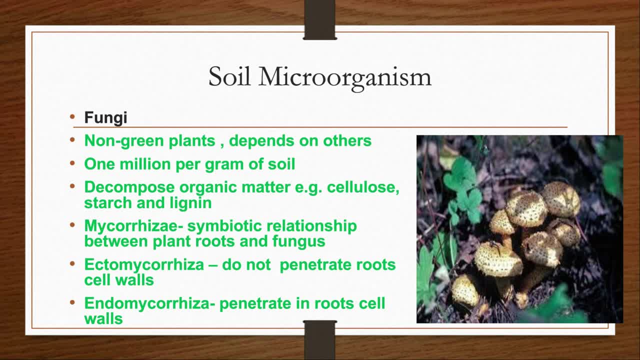 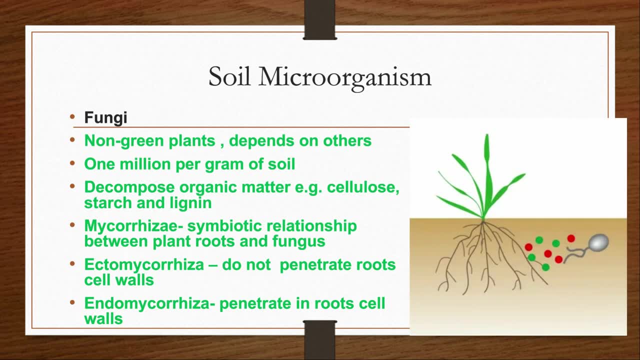 In return, fungi provide essential nutrients, including phosphorus, to the plant and and help plant to uptake water, While mycorrhizae are divided into two types: ectomucurrhiza and endomucurrhiza. in ectomucurrhiza, hyphae fungi penetrate the root of plant but do not penetrate cell wall. 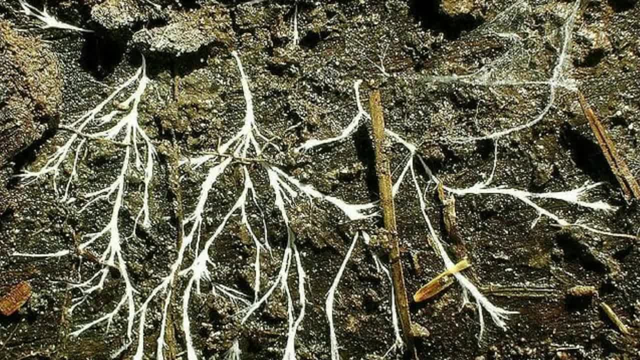 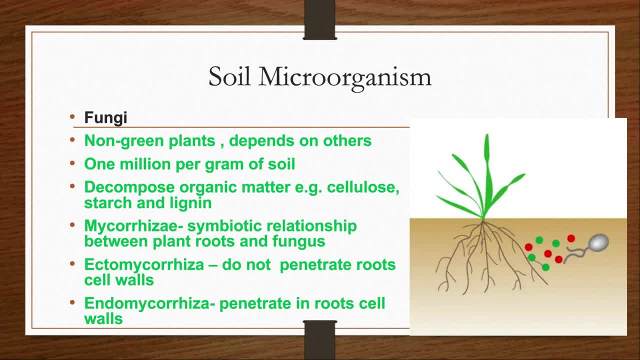 actually hyphae are long branching, Fragmented structure of fungus, of mycorrhiza association mostly with trees such as oak tree. while in endo mycorrhizae- that is also called a vesicular or vascular mycorrhizae, penetrates roots of the cell wall, about 90% of our plants, including wheat cotton. 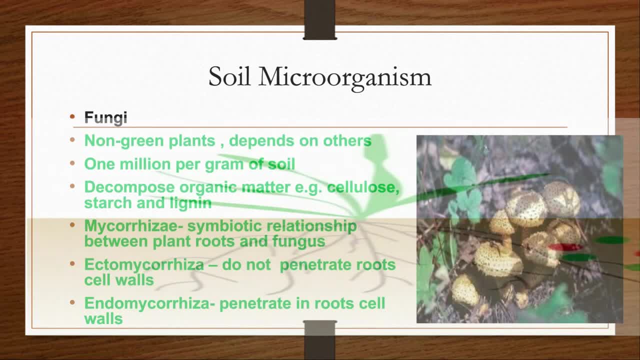 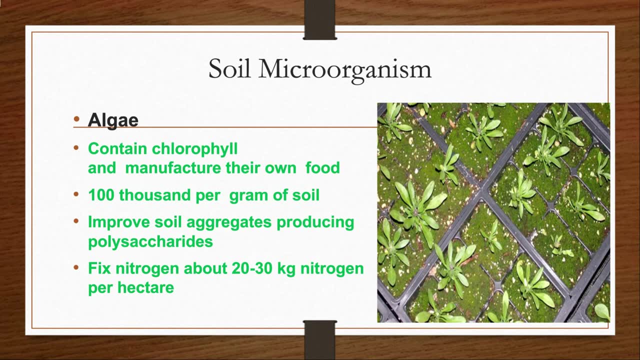 sugar have endo mycorrhizae association algae. algae is also soil microbes. they contain chlorophyll and they manufacture their own food, like plant, while one gram of soil contain hundred thousand algae. algae is good for soil structure. they improve soil aggregate by producing polysaccharides, while in 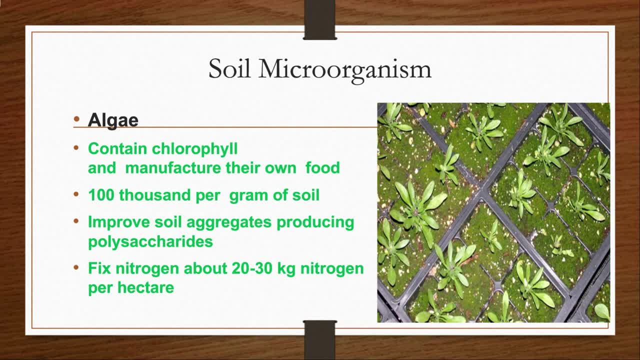 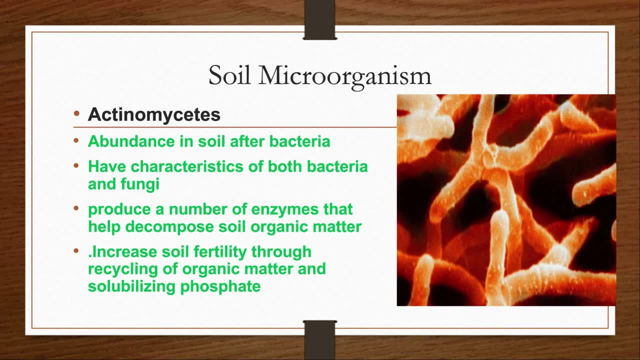 waterlogged rice field algae fix about 20 to 30 kg nitrogen per hectare. actinomycetes: actinomycetes are abundance in soil after bacteria. actinomycetes are abundance in soil after bacteria. actinomycetes are abundance in soil after bacteria. 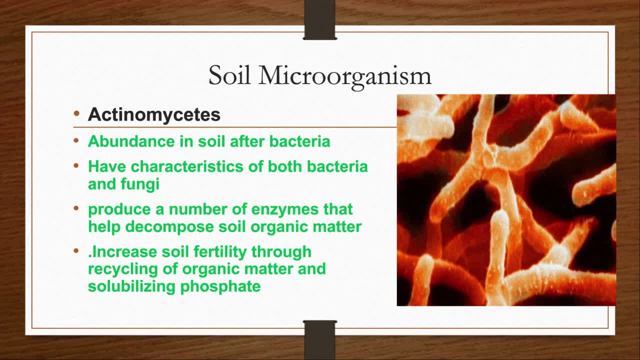 and they have characteristics of both bacteria and of fungi. they produce number of the enzymes that have to decompose to soil organic matter. the actinomycetes increase soil fertility through recycling of soil organic matter and solubilizing phosphate if phosphorus is insoluble in soil that is unavailable. 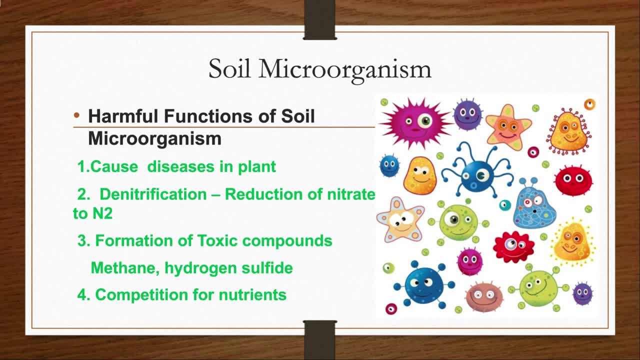 for the plants. harmful functions of soil microorganisms. microbes present in soils are very important for soil, but they have some harmful functions as they cause diseases in plants. like disease of rice is caused by bacteria, and fungi cause many diseases, including summers and a rust of a cereal crops, while denitrifying.